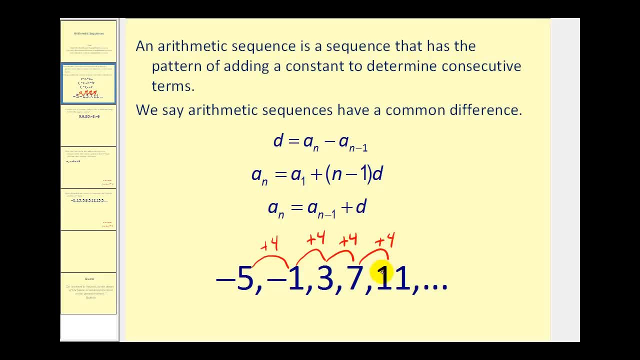 stays consistent of adding a constant, this is an arithmetic sequence. And what we'll notice is we can find the common difference from this formula by selecting any term in the sequence and subtracting the term before it. So if we use a sub two, we would subtract a sub one. Negative one minus negative five will give us positive four. If we want to use the fifth term in the sequence, we would have to subtract the fourth term. Eleven minus seven also equals positive four. This next formula a sub n equals a sub one 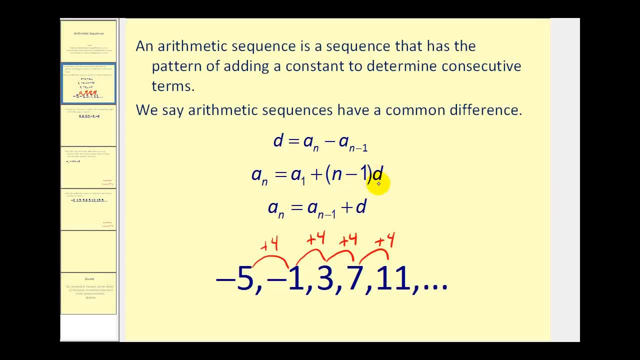 plus n minus one times the common difference, you might be thinking why the n minus one? 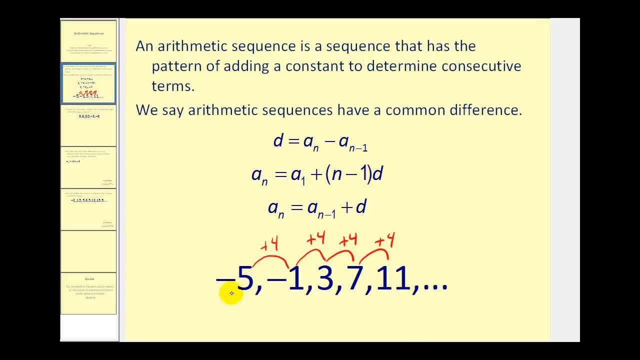 Well if you take a look at the sequence again and look at the pattern, notice the second term we added four one time. The third term we would add four two times. And the fourth term we would add four three times. So we'll always add n minus one 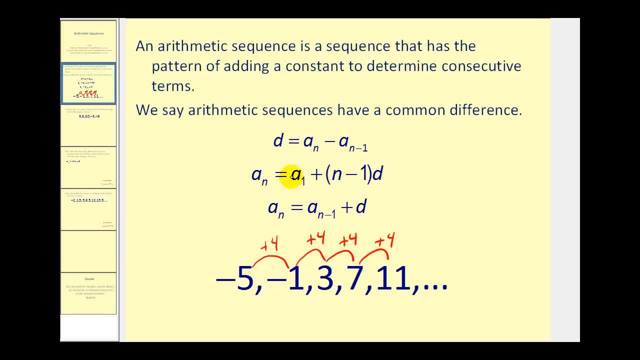 multiples of the common difference to the first term to get any other term in the sequence. And this last formula here is a recursive formula, which just means 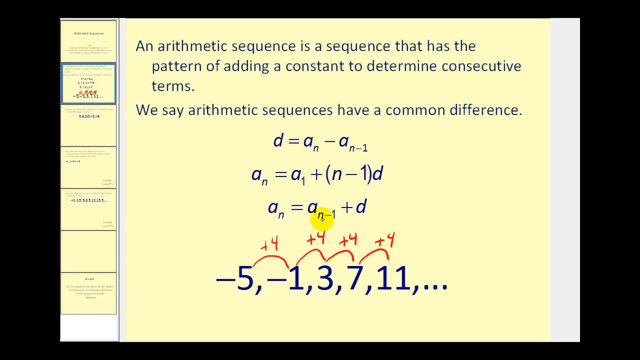 if we want to find, let's say the fifth term, we just take the fourth term, a sub n minus one, and then add the common difference. And this is just emphasizing 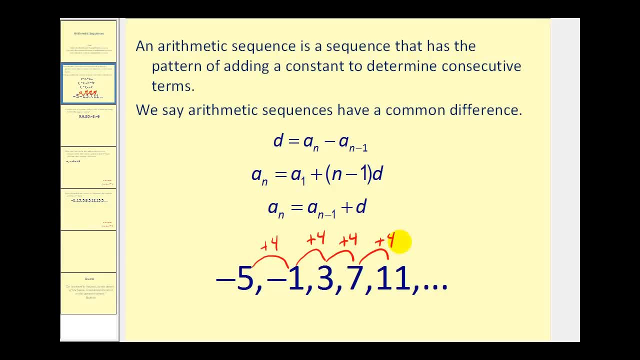 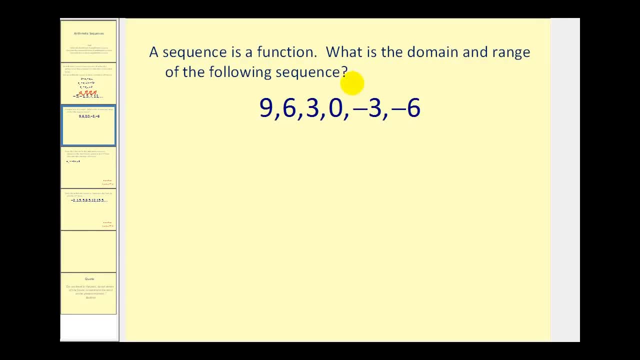 the pattern that we see here in red. Let's go ahead and see if we can answer some questions using arithmetic sequences. Again as we stated in the previous video, a sequence is a function. So we can identify the domain and the 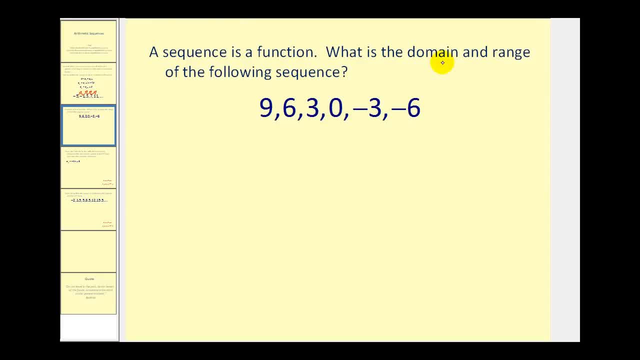 range. And what's helpful to determine the domain and range is to label each term as a sub one, a sub two, a sub three, a sub four, a sub five, and lastly a sub six. So the values of n represent the domain. So the 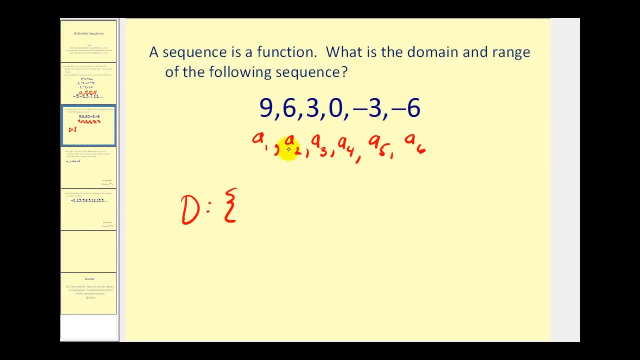 domain of this sequence will be one, two, three, four, five, and six. 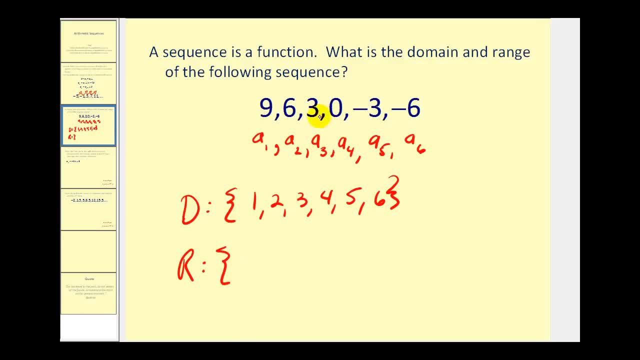 And the range of the sequence would be the actual elements in the list. And we usually list these from least to greatest. So we'll list the range as negative six, negative three, zero, three, six, and nine. 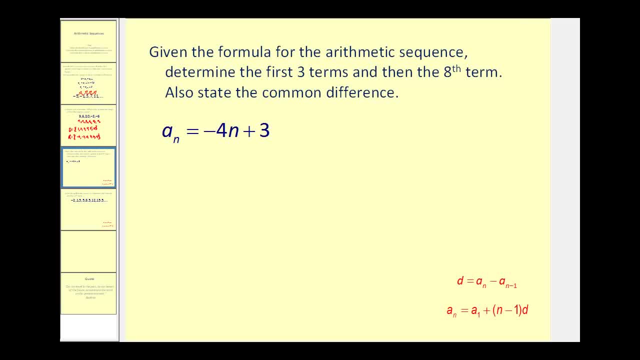 Okay on this problem we're given the formula for the arithmetic sequence. We want to determine the first three terms and then the eighth term. So we want to find a sub one, a sub two, a sub three, and a sub eight. So if we want a sub one, that means n is equal to one. So we have negative four times one plus three. That's negative one. A sub two, that means n is equal to two. Negative four times two plus three. Negative eight plus three is equal to negative five. A sub three, so n is three. We have negative twelve plus three, that's negative nine. And the eighth term, that means n is equal to eight, negative four times eight plus three. We have negative thirty-two plus three, that's negative twenty-nine. So the sequence would look like this. 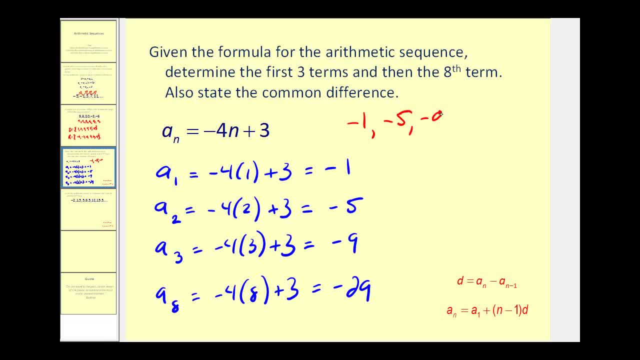 Negative one, negative five, negative nine. 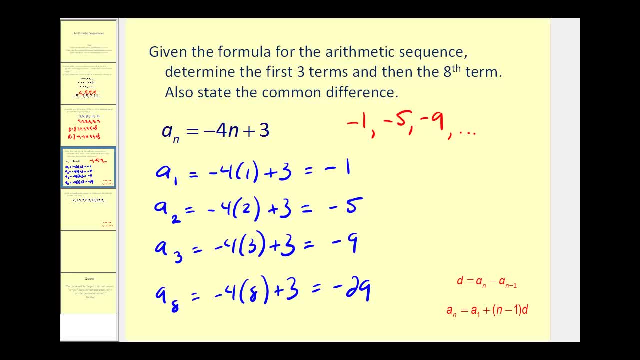 Then the eighth term would be negative twenty-nine. They also asked us to state the common difference. Remember to find the common difference, 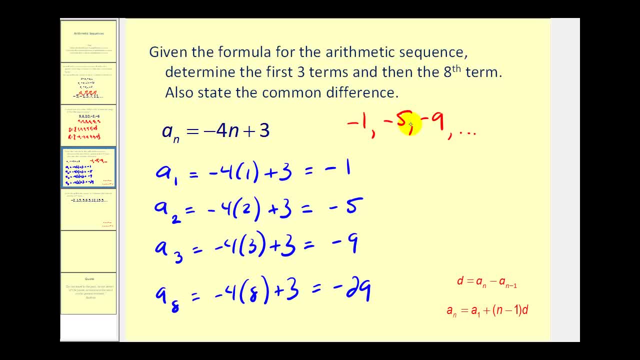 we just select one term and then subtract the term before it. So if we use a sub two, the common difference will be negative five minus a sub one, which is negative one. So we have negative five plus one, so the common difference is negative four. 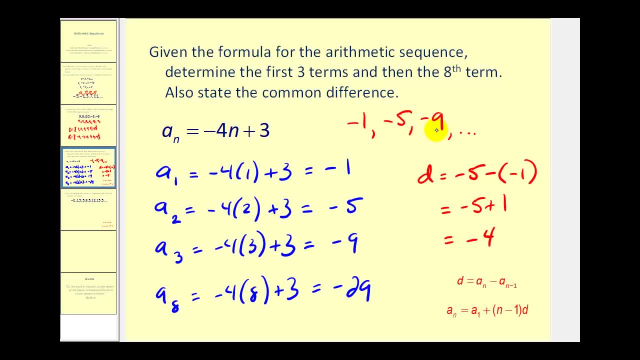 And we can see this sequence is decreasing by four each time because we're adding negative four each time. Let's go and take a look at this question now. 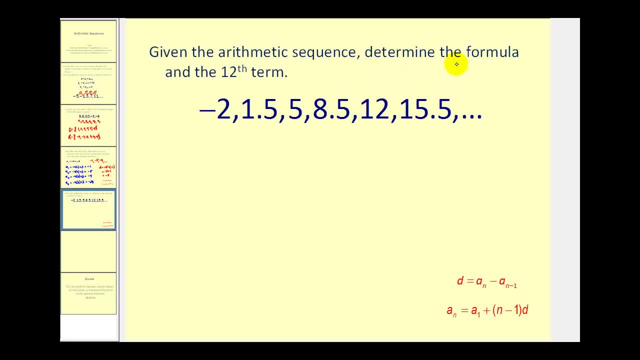 We're given that it's an arithmetic sequence. We want to determine the formula for the sequence and then also determine the twelfth term. To determine the formula for the sequence, we're going to have to determine the formula for a sub n as we see here. So we're going to have to find a sub one and also the common difference to use this formula. So let's go ahead and write this out. A sub n equals a sub one plus n minus one times d. A sub one is the first term, so a sub one equals negative two. And to determine the common difference, we're going to select any term and then subtract the term before it. So if I wanted to use the term here that's equal to twelve, the common difference would be twelve minus the term before it, or eight point five. 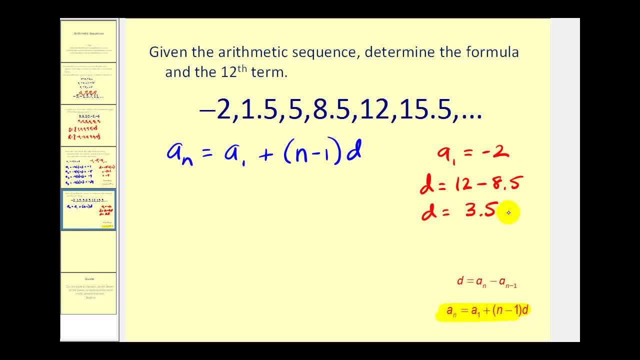 So the common difference is equal to three point five. Remember I can obtain the common difference by selecting any term and subtracting the term before it. So if I wanted to use this term here, one point five minus negative two is still going to equal three point five. Now that we have a sub one and d, we can substitute those values into the formula and find a sub n. So a sub n equals negative two plus n minus one times the common difference of three point five. 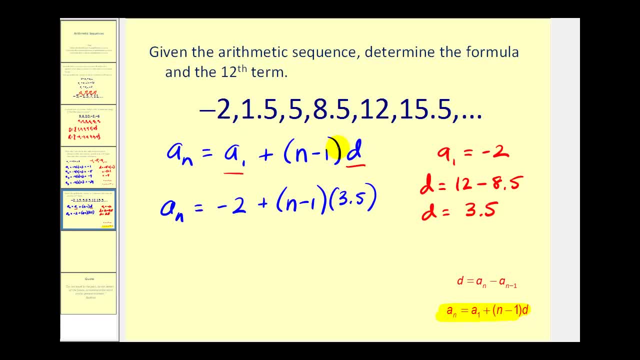 Now this is the formula to determine any term in this sequence, but normally we'll be asked to simplify this. So we'll distribute three point five and then combine any like terms. So we'll have a sub n equals negative two plus three point five n minus three point five. Here we have two like terms, so our formula will be a sub n equals three point five n minus five point five. 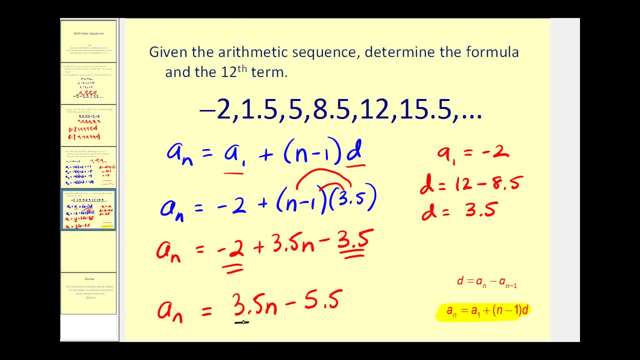 One more thing to notice here, if you take a look at the coefficient of the n term, it is equal to the common difference. 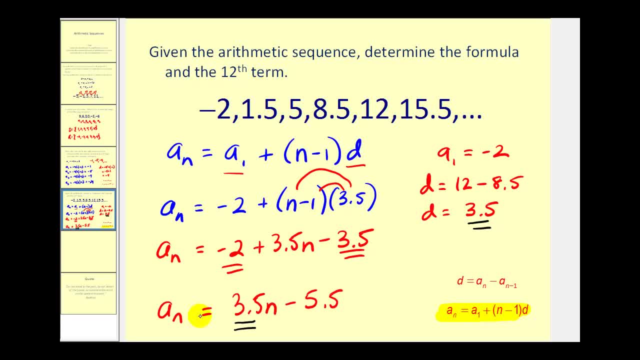 We were also asked to determine the twelfth term, so using this formula we'll let n equal twelve to find that twelfth term. Let's go ahead and do that on the next slide.